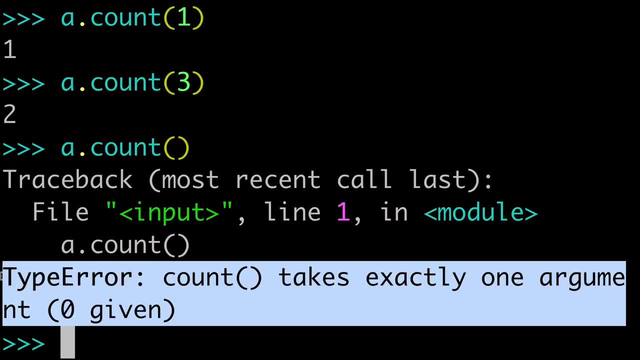 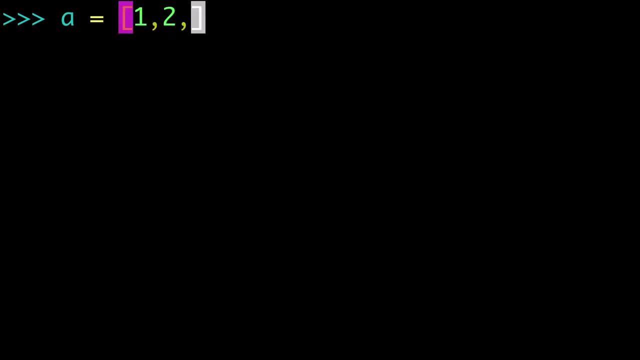 1 here that has two occurrences right. So if I pass 1 here that has two occurrences right, We'll get a type error saying that the count takes exactly one argument. So let's start building up our list to something a little more complicated. to show you a few more examples. So 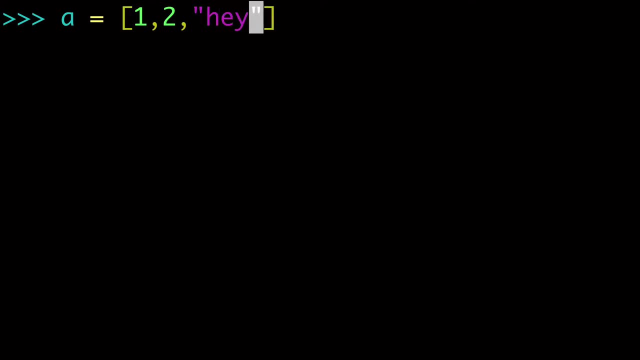 here I'm working with numbers, but we could also do strings. We could also do a list nested inside our list. So I don't know, I'll call this nested. We could also do a dictionary and I'll just put a quick key value pair here. So now we have a string, a list, a dictionary. 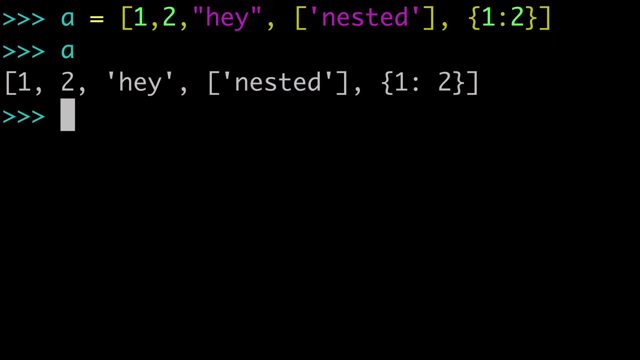 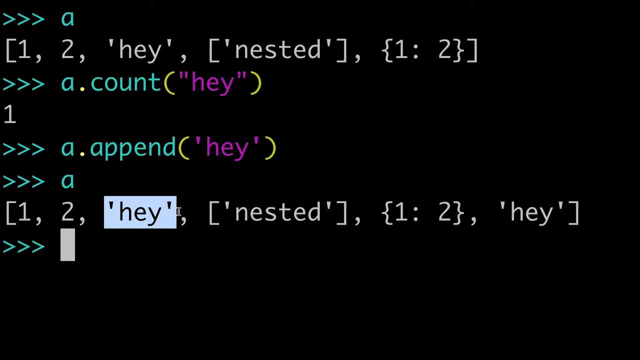 as well as some integers, And that is a. that is our list. So how could we check the count Again? we do a dot count And then I could check the occurrences of hay in this list And if I did a dot append and I added another hay onto it, we could. we can check our our list, a again. So now, 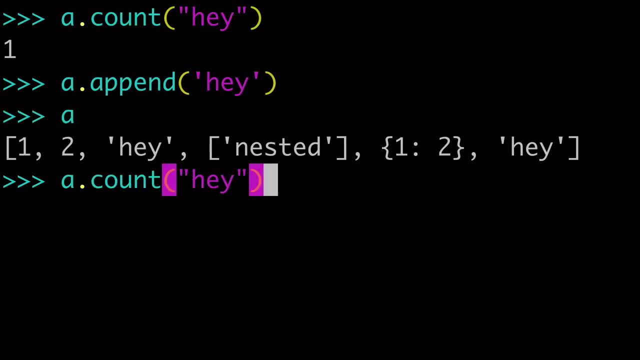 we have two hayes And when I go to run that count again, we can see that we have two hayes. Again we get two. So it's taking into account that we have added another one. you know, obviously counting both of our string values, And what I really wanted to get across here is that you don't 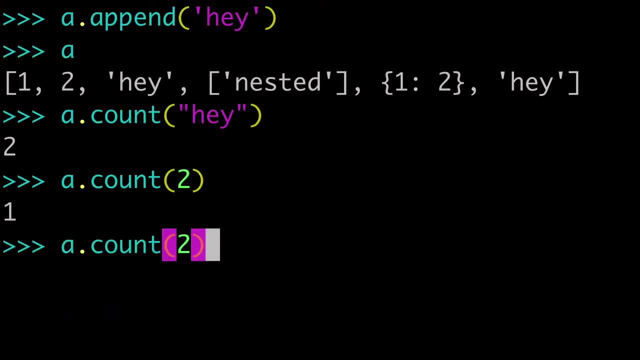 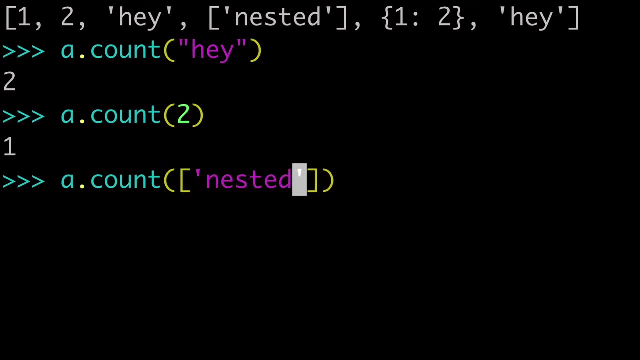 just have to pass numbers, right. So of course we can pass numbers. Now we know we can pass strings and we can of course, even pass a list in here. So I think I had a list that said nested in here, right. So we had one occurrence of that. We also had a dictionary in there, so I can pass our. 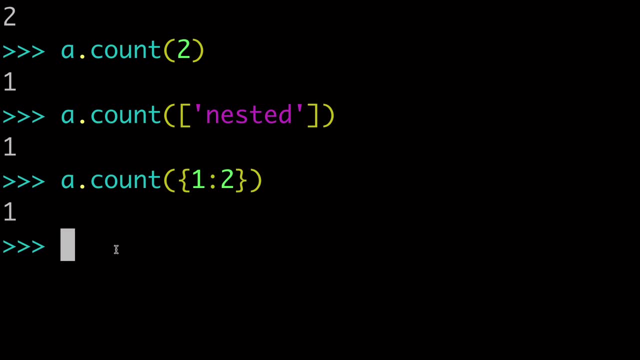 dictionary Right in there and we're getting a value. Of course, if we pass, say, an empty dictionary or an empty list, we're going to get zero because we don't have any empty dictionaries, we don't have any empty lists. So pretty intuitive, pretty straightforward. That is the basics of how to. 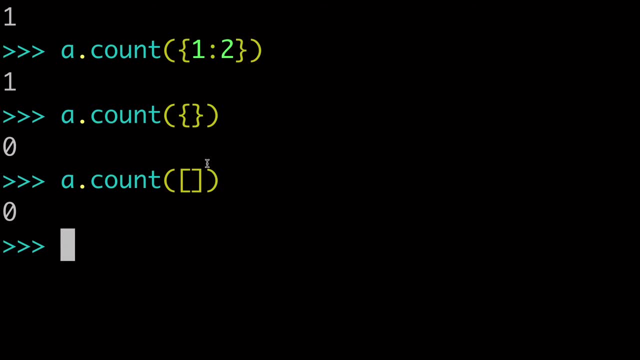 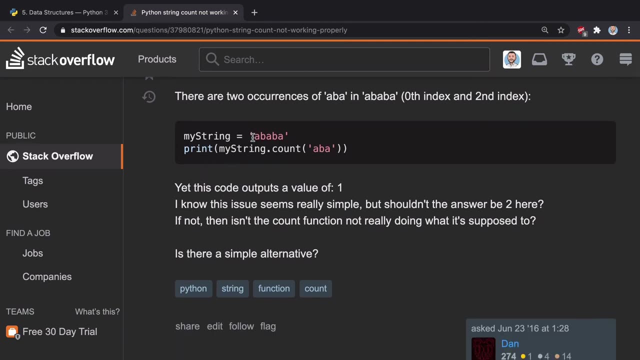 work with the count list method. The other thing I really wanted to show you guys- I think is well highlighted in this stack overflow post- And basically what this guy is trying to do is he's saying that there's two occurrences of aba n a ba ba right, So these would have to overlap.